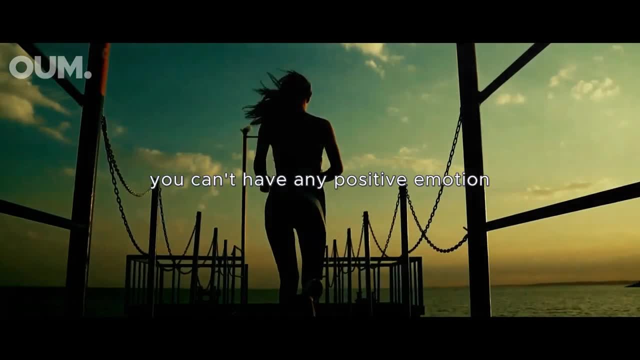 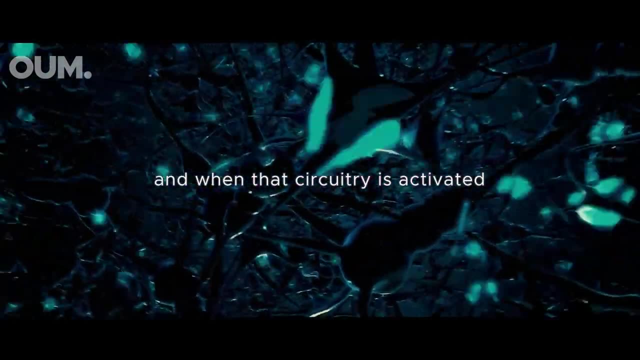 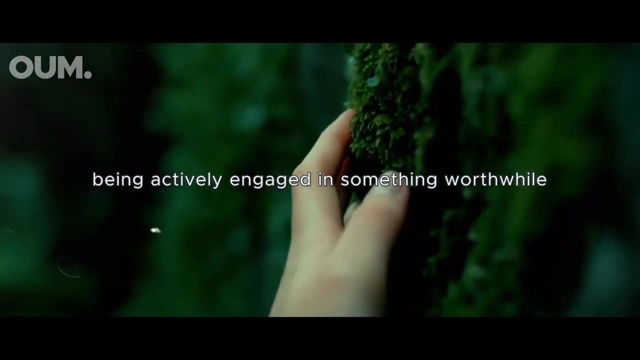 And so that means that if you don't have a goal that you value, you can't have any positive emotion. So technically that's the incentive-reward system, and the underlying circuitry is dopamine. When that circuitry is activated, then it's part of the exploratory circuit. It gives you the sense of being actively engaged in something worthwhile. 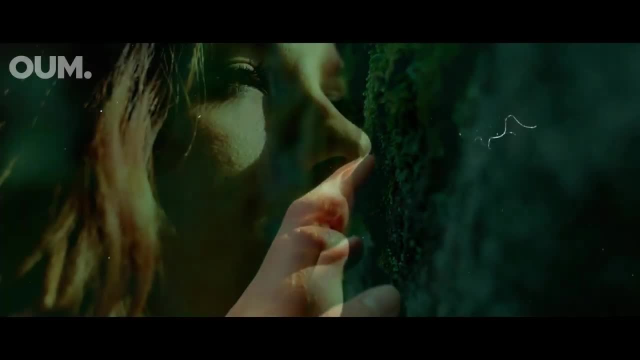 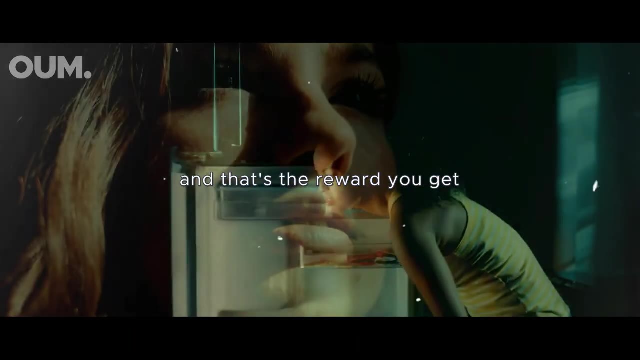 You tend to think of positive emotion as something produced by reward, but there's two kinds of positive emotion. One is the reward that's associated with satiation and that's consummatory reward, and that's the reward you get when you're hungry and you eat. 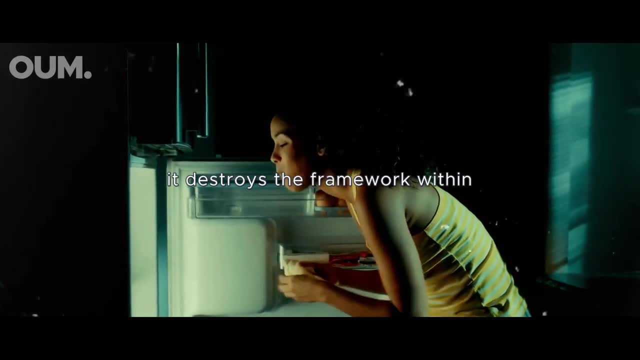 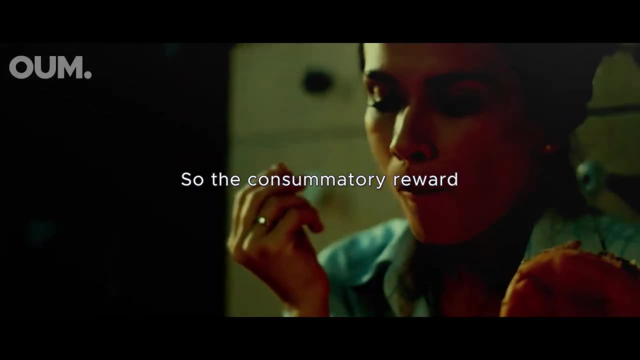 But the thing about eating when you're hungry is that it destroys the framework within which you are eating Operating. but it's time to eat while you eat, and then that frameworks no longer relevant. so the consummatory reward Eliminates the value framework, and then you're stuck with well. 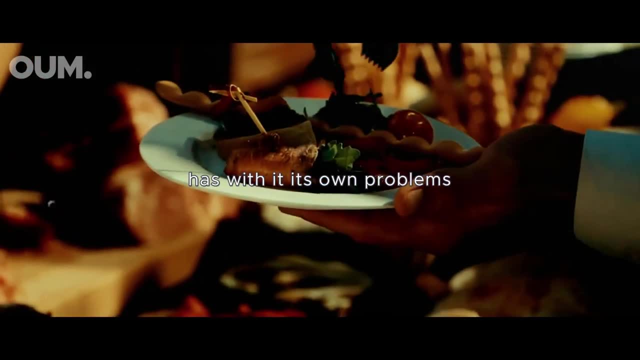 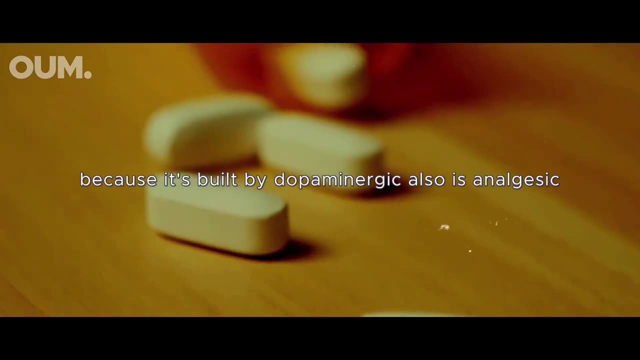 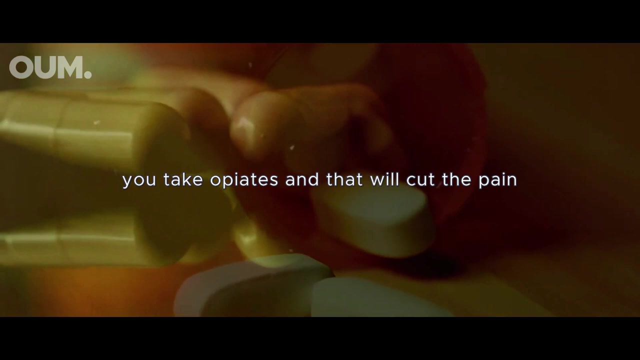 What are you going to do next? and so the consummatory reward has with it its own problems, but the incentive reward is constantly what keeps you moving forward. and Incentive reward, because it's dopaminergic also, is analgesic, Literally analgesic. so if you're in pain, you take opiates and that that will cut the pain. 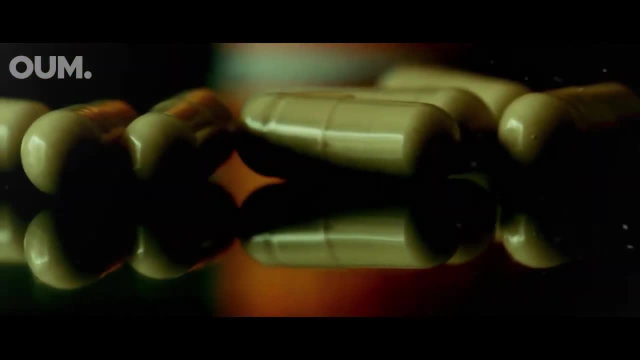 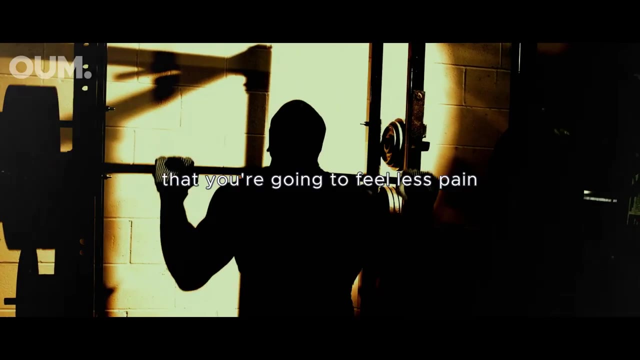 but so will psychomotor stimulants like cocaine or amphetamines, and So it's literally the case that if you're engaged in something That's engaging and you're working towards a goal, that you're going to feel less pain, And you can see this happening with athletes who you know. 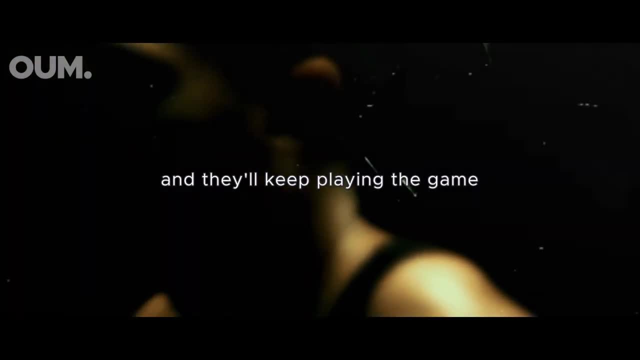 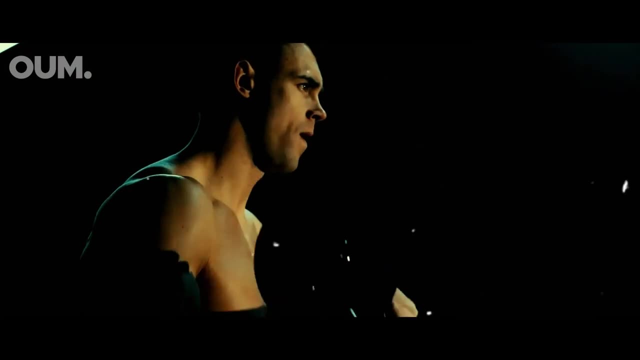 They'll break their thumb or something, or maybe sometimes even their ankle, and they'll keep playing the game. of course, afterwards They're suffering like mad, but the fact that they're so filled with goal-directed enthusiasm means that, Well, the pain systems are in some sense shut off. 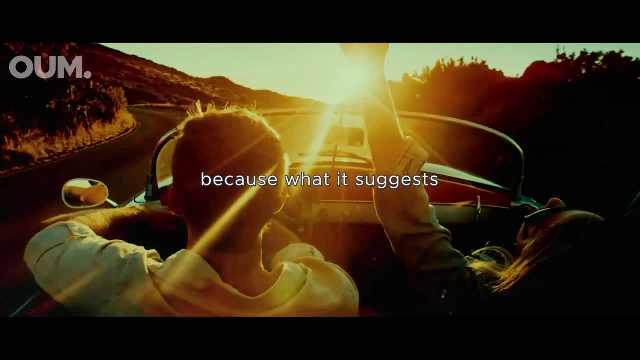 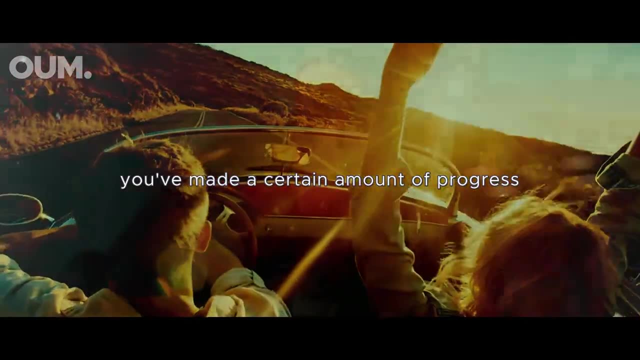 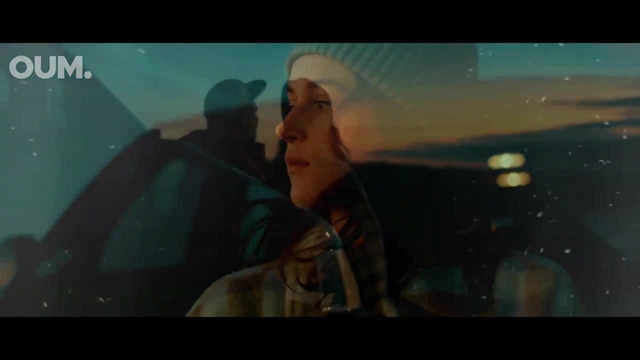 So that's an interesting thing, because what it suggests, I mean, then you could imagine, I might say well, How happy you are, you that you've made a certain amount of progress. and if you think about it, what you'd say is: well, It depends on how much progress and in relationship to what. so hypothetically, you're going to be happier. If you've made quite a bit of progress towards a really important goal.